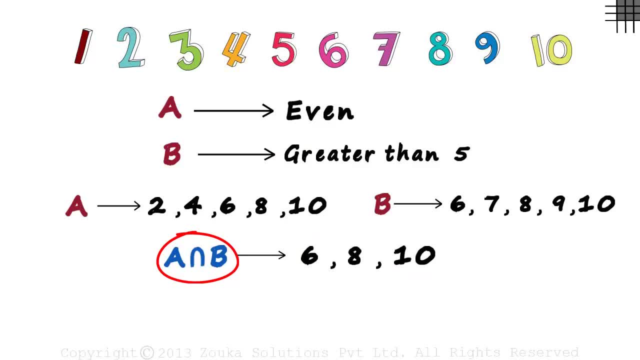 So what will be the probability of events A and B happening together? Three numbers out of a possible ten. So the probability of both events, A and B, happening together, will be three by ten. This also equals zero point three, or thirty percent. In layman terms, we can say that there is a thirty percent chance. 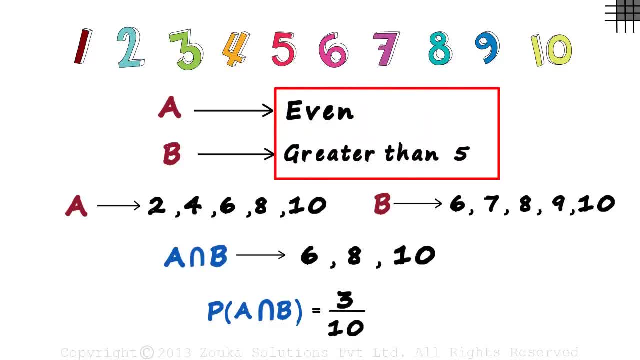 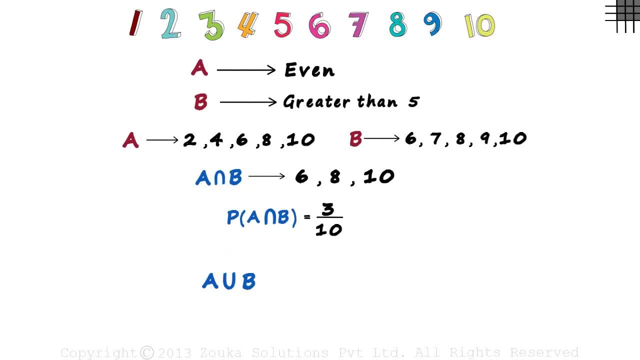 of picking up a number that is even and greater than five. Let's zoom out and see what A union B will be equal to. This is interesting. It means either getting an even number or a number greater than five, Or a number which is both even and greater than five. 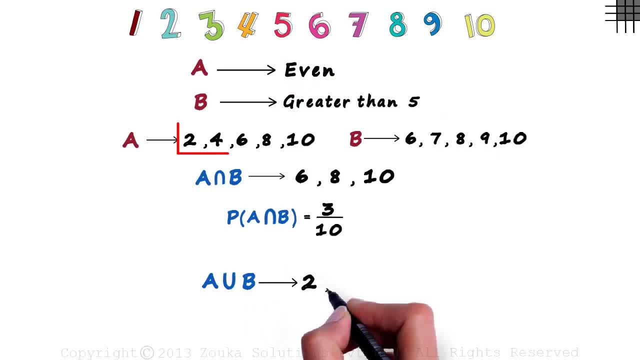 So let us note the even numbers first. Two, four, six, eight and ten are the even numbers. We also need to jot down numbers greater than five. Six is greater than five, But it's already included in the even numbers list. 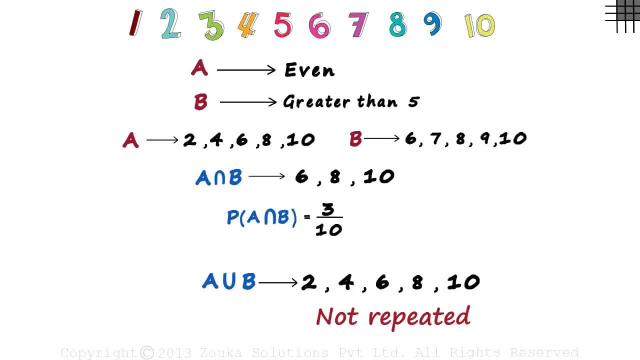 So we don't write it down. Remember, numbers should not be repeated. The next number greater than five is seven, And that is not written, So we write a seven. Similarly, eight and ten are already included. What remains is nine. 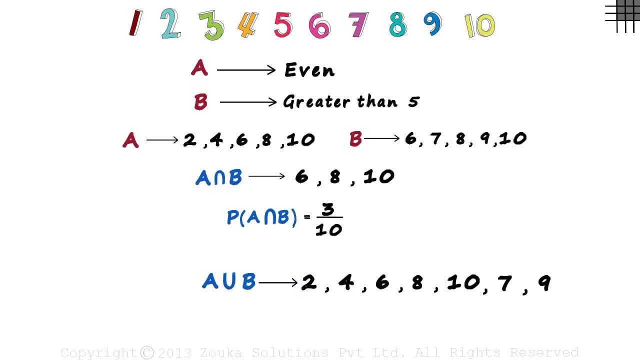 So these are the possibilities of event A or B happening, Seven in all. No matter what number we pick from this set, it will surely be either Even or greater than five, Or it is possible that our pick is both even and greater than five. 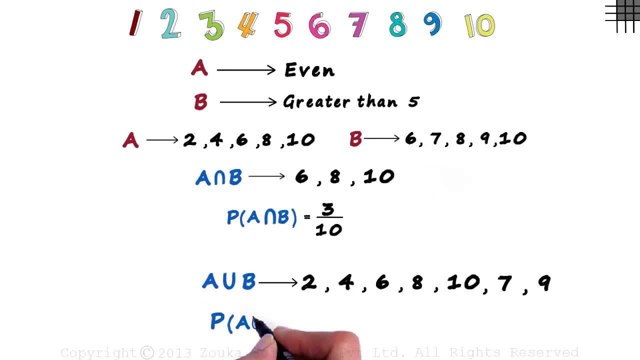 What we are interested in is probability of A or B. There are seven numbers here out of a possible ten, So the probability of A or B happening is seven divided by ten. If you look at this set carefully, you will see that it contains numbers only belonging to A. 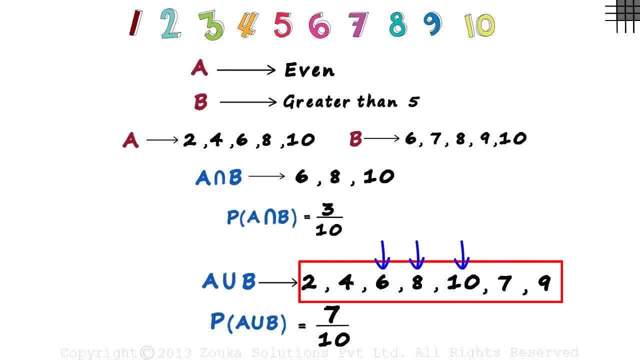 only belonging to B, and belonging to both A and B. Since this was a small set of numbers, we could use this method of looking for numbers manually, But for a bigger set we may have to use a formula In the coming videos. 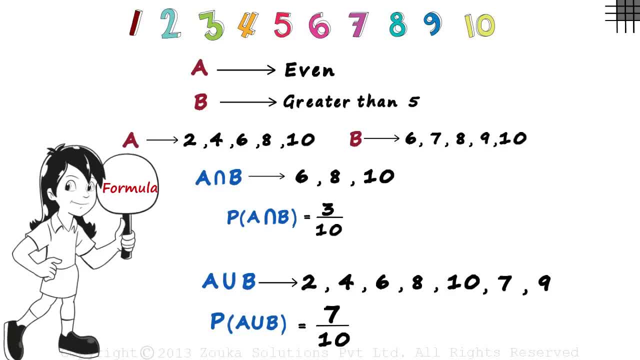 we will see how formulae can be used to find such probabilities.